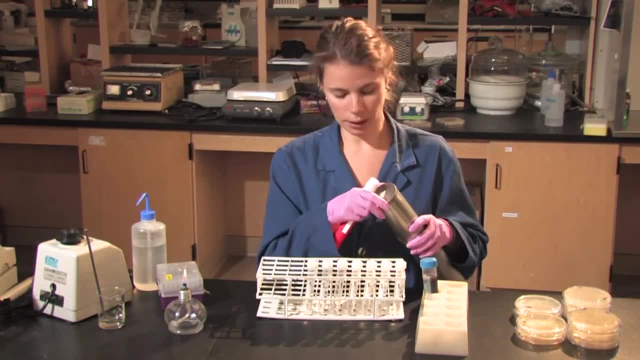 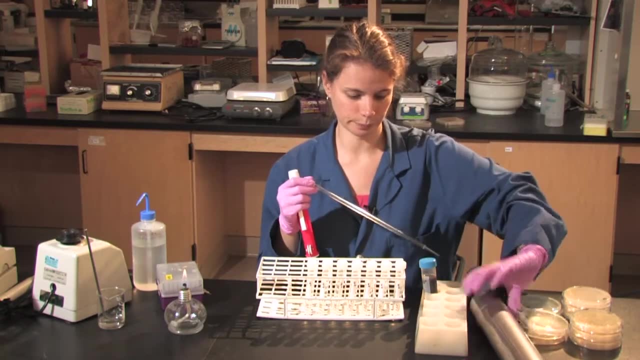 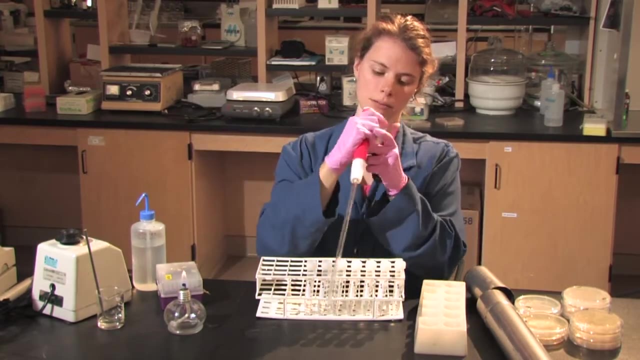 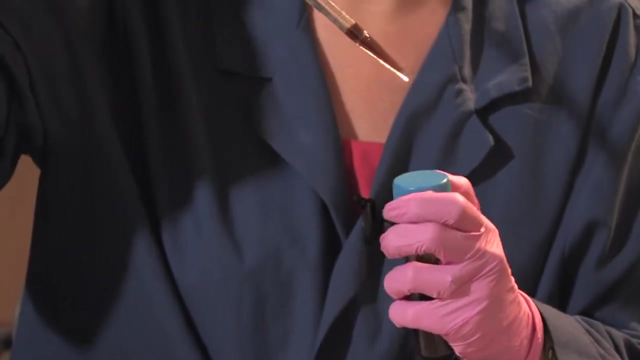 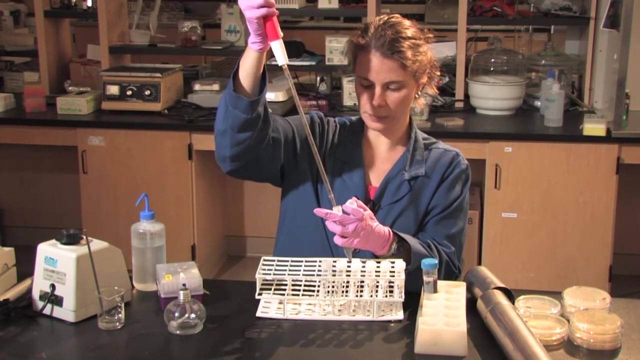 but to make it easier for us to visualize, I'm doing it here. So I've got my autoclaved pasteur pipettes and I'm going to add one mil of the soil- 10 to the zero soil solution- to nine mils of distilled water, and this gives me a 10 to the minus one dilution. 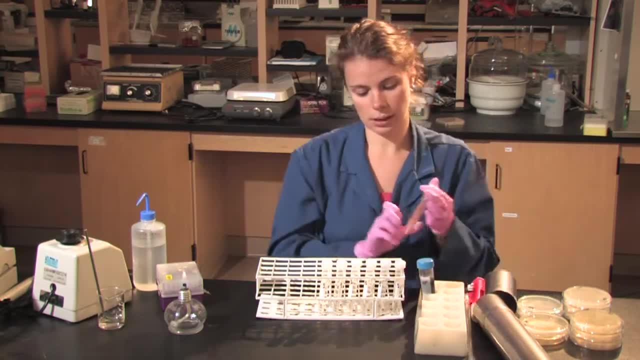 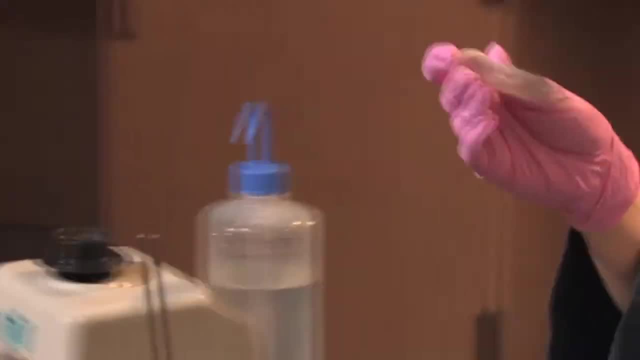 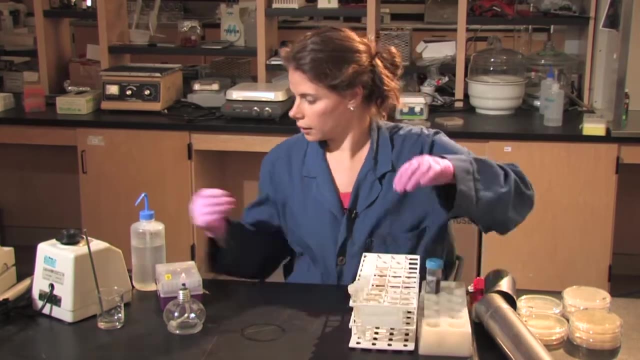 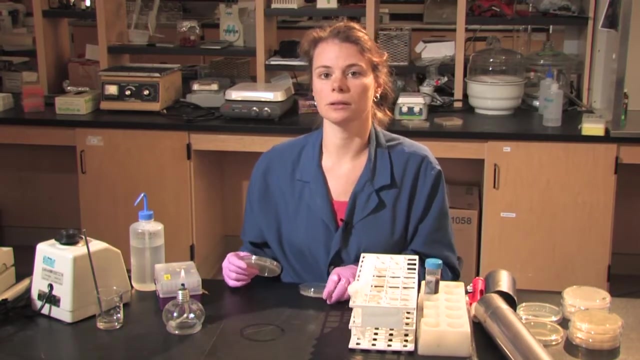 And I would continue along in this nature until I get to 10, to the minus seven. I then vortex each dilution again, distributing the sample. I'm then going to plate on two different types of agar: a potato dextrose agar, which is for fungal growth, and then we've got a tryptic soy agar. 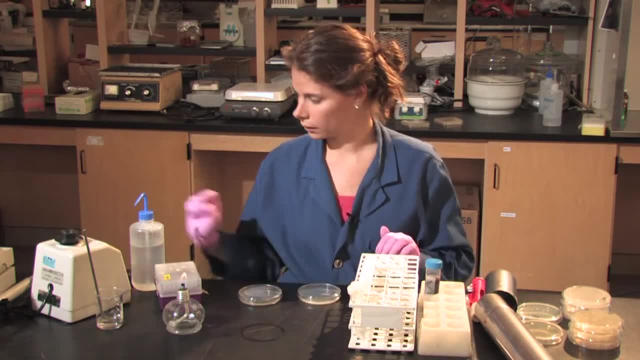 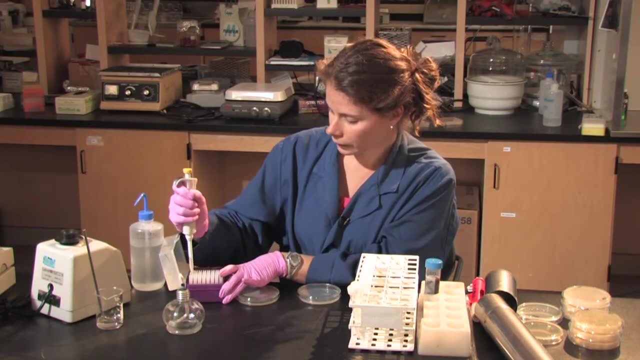 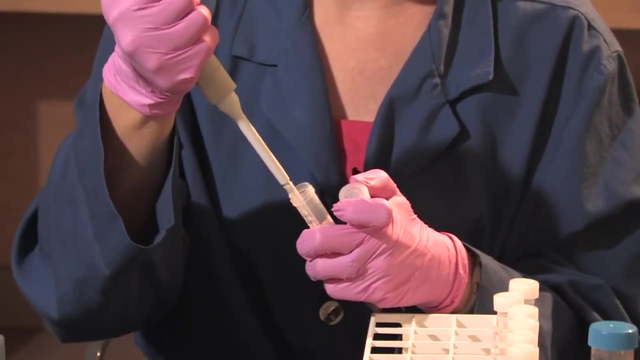 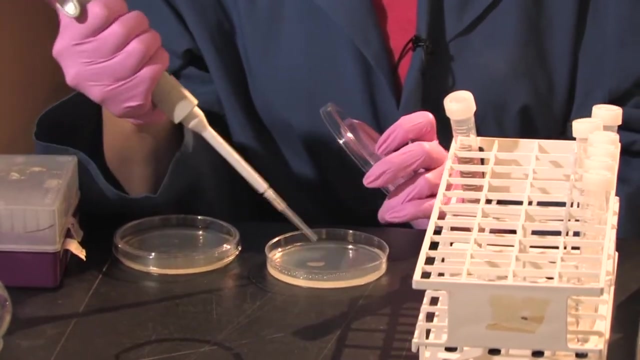 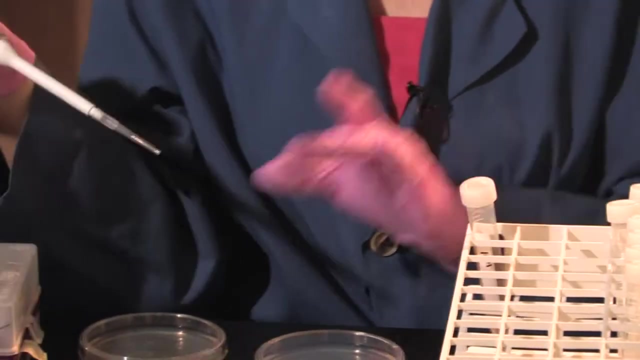 which is for bacterial growth. I have my micropipetter which is set at a hundred microliters and I'm going to add hundred microliters of the 10 to the minus 1 dilution to each plate And to the triptych soy agar plate. 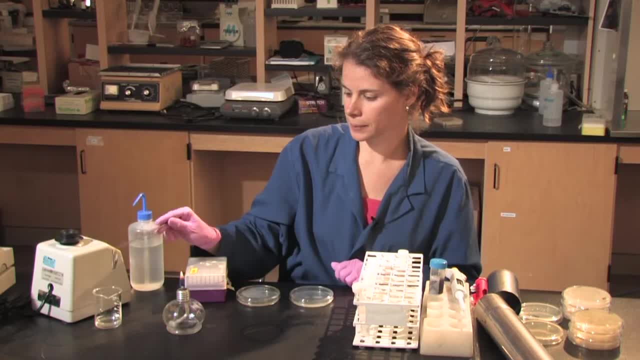 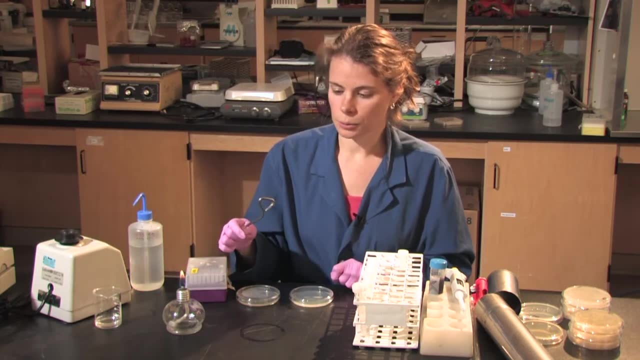 I have a spreader here in ethanol and I will put it through the flame. This burns off the ethanol and aseptically well sterilizes my spreader between samples so that I don't have any contamination, Because I don't have any contamination. 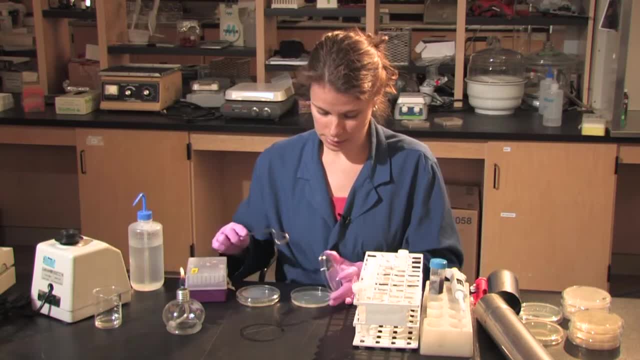 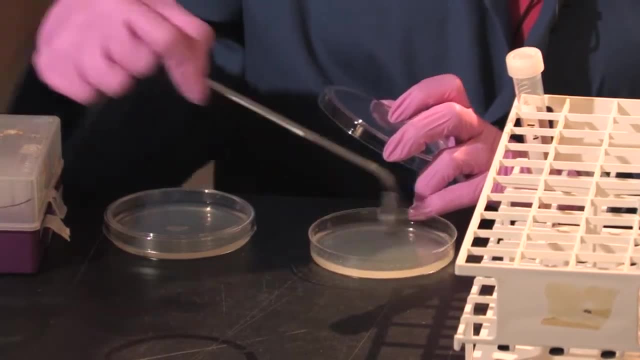 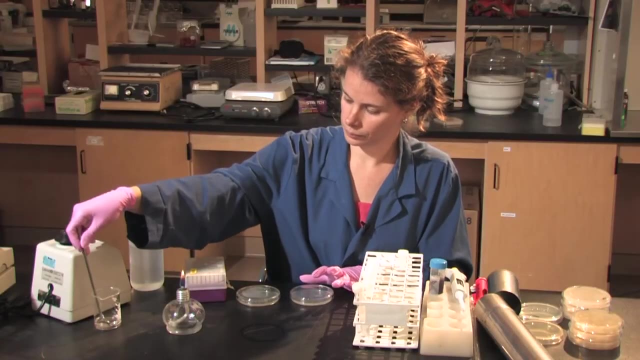 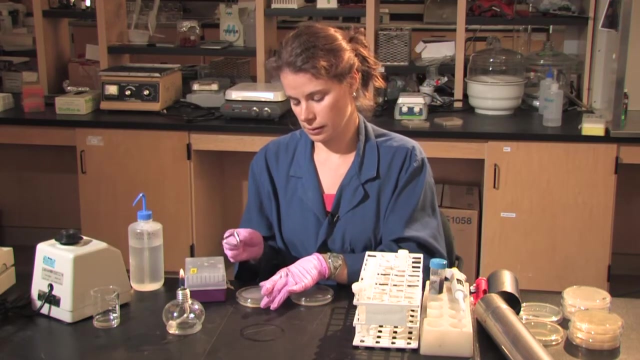 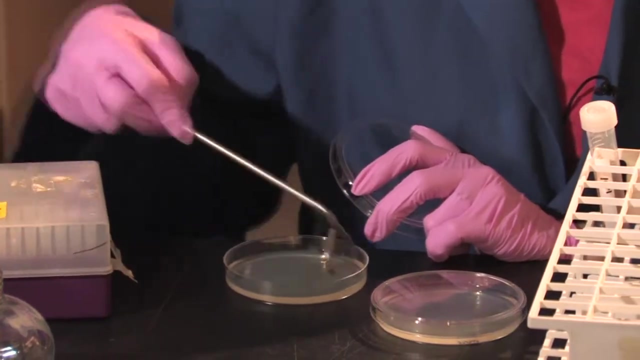 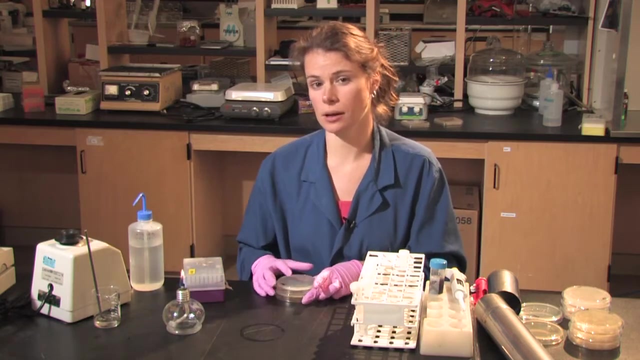 Between the samples or from outside sources. Once my spreader's cooled, I will put it through the hundred microliters of the solution, distributing it evenly across the plate. Do the same for the second plate. Once the solution is spread evenly, I will flip the plates so as not to get any moisture.